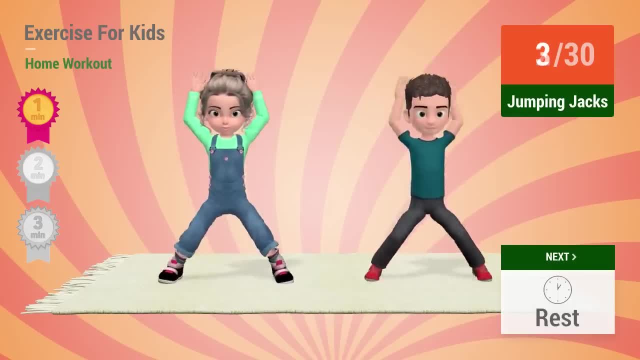 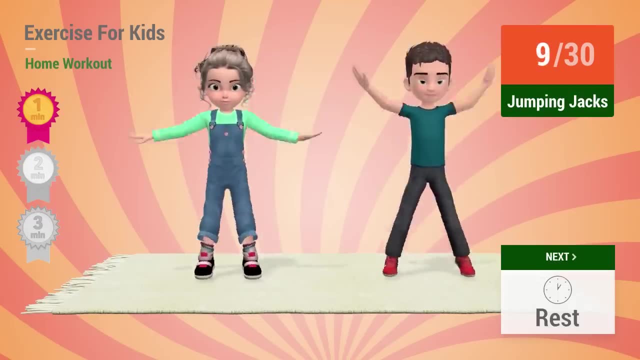 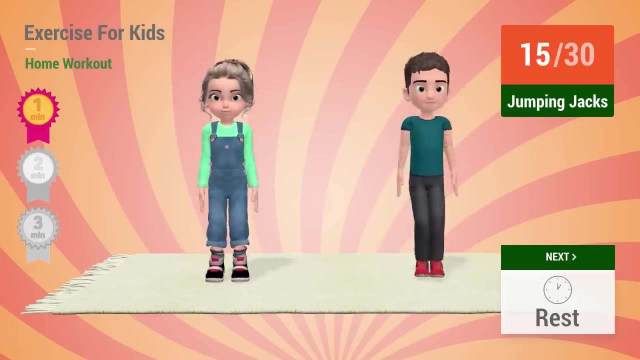 1,, 2,, 3,, 4,, 5,, 6,, 7,, 8,, 9,, 10,, 11,, 12,, 13,, 14,, 15,, 16,, 17,, 18,, 19, 20.. 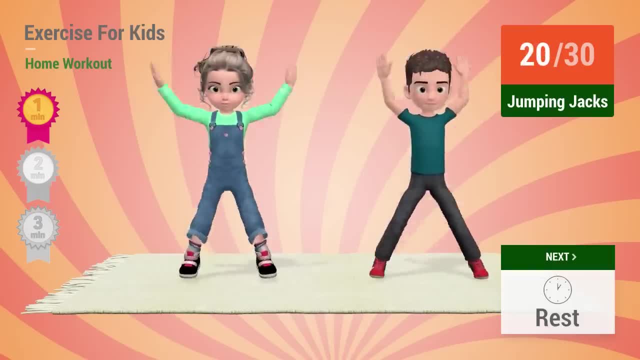 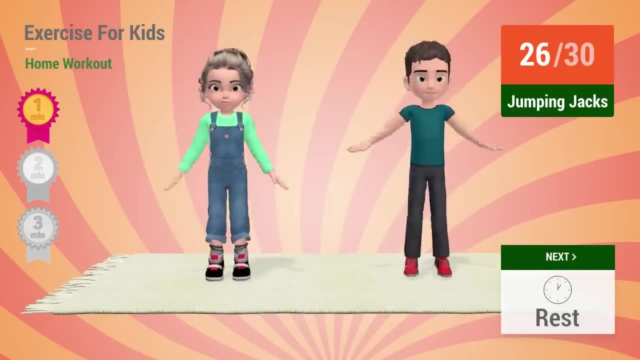 Up next jumping jacks in 5,, 4,, 3,, 2,, 1.. Go Up next jumping jacks in 5,, 4,, 3,, 2,, 1.. Go 17,, 18,, 19,, 20,, 21,, 22,, 23,, 24,, 25,, 26,, 27,, 28,, 29,, 30. 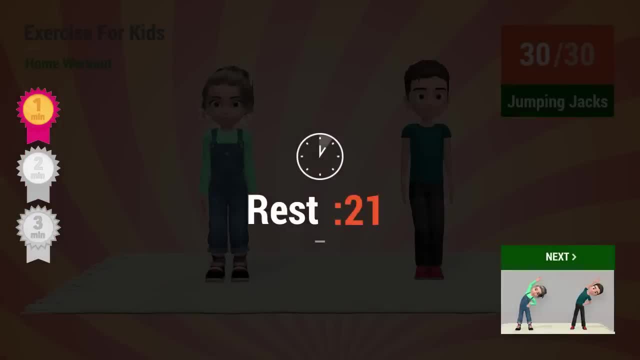 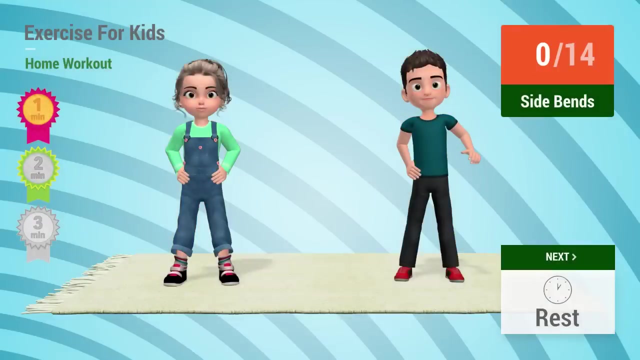 Rest time. Good work, You're working out for two minutes already. Let's continue Up. next side bends in 5, 4,, 3, 2, 1.. Go 1,, 2,, 3, 4, 5.. 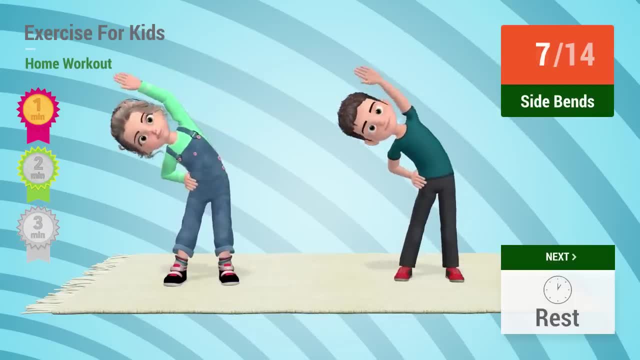 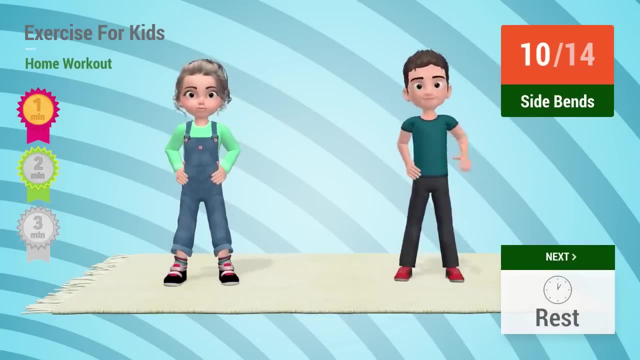 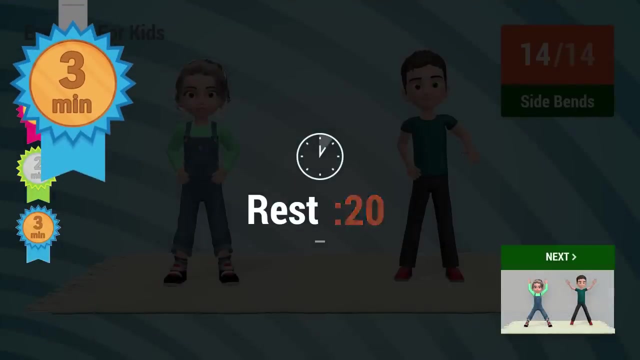 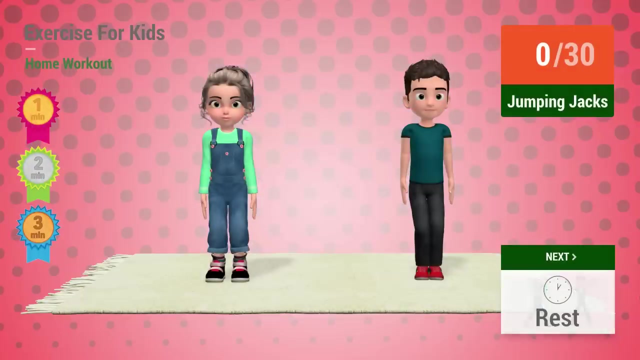 6,, 7,, 8,, 9,, 10,, 11,, 12, 13, 14.. Rest time: You're three minutes in Good job and keep exercising Up. next, jumping jacks in 5,, 4,, 3,, 2,, 1.. 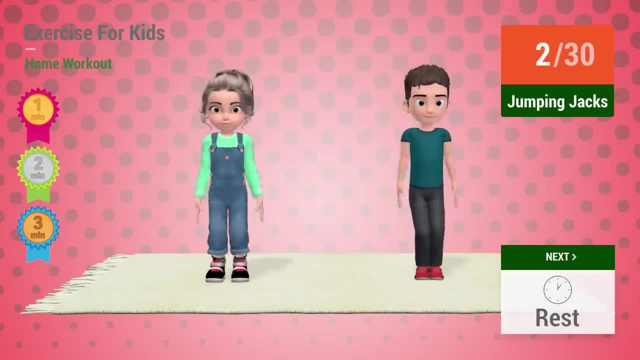 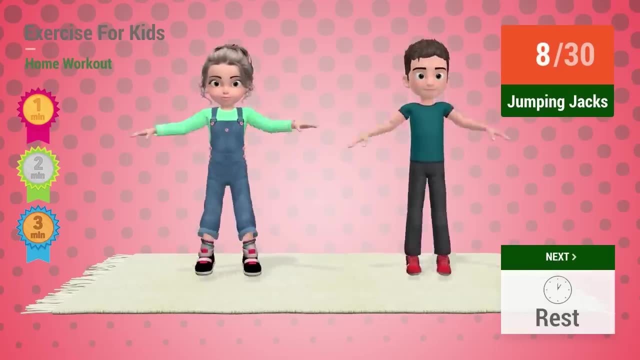 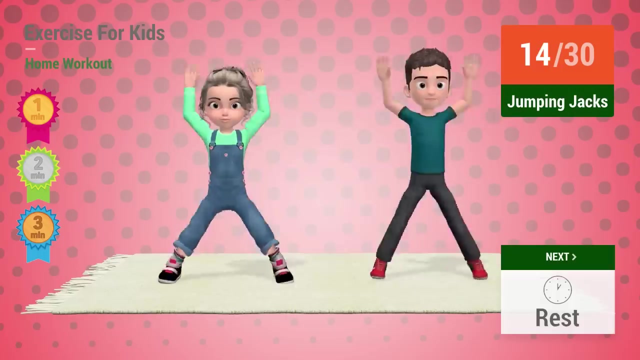 Go: 1,, 2,, 3,, 4,, 5.. 6,, 7,, 8,, 9,, 10,, 11,, 12,, 13,, 14.. 6,, 7,, 8,, 9,, 10,, 11,, 12,, 13,, 14,, 15,, 16,, 17,, 18,, 19,, 20,, 21,, 22,, 23,, 24,, 25,, 26,, 27,, 28,, 29,, 30. 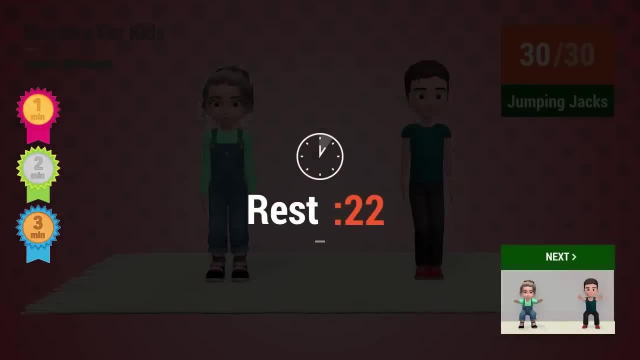 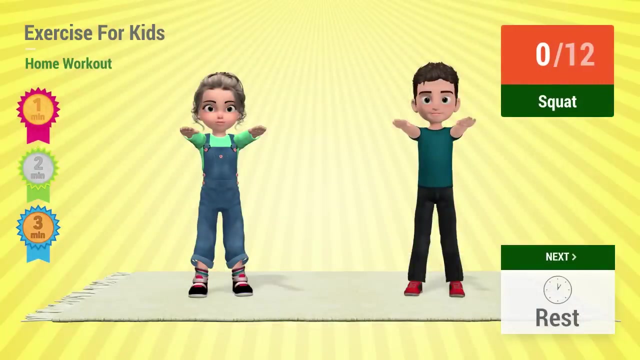 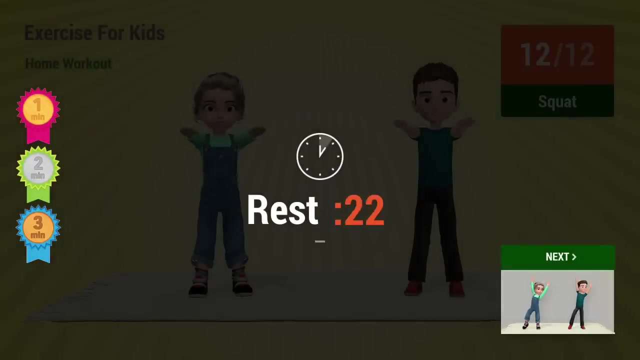 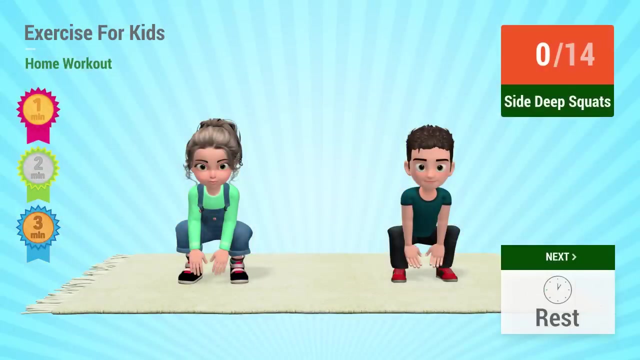 Rest time. You're three minutes in. Up next squat in 5, 4, 3, 2, 1.. three, two, one go one. two, three, four, five, six, seven, eight, nine, ten, eleven, twelve rest time. up next side deep squats in five, four, three, two, one go one. 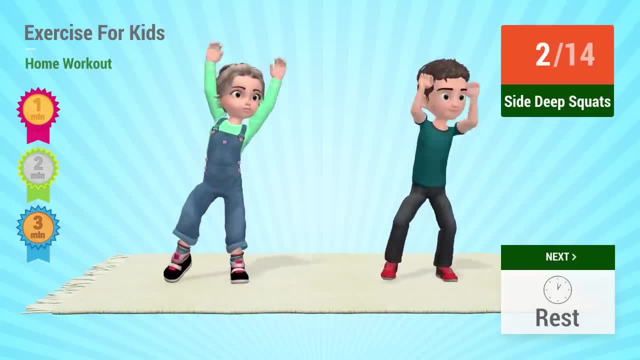 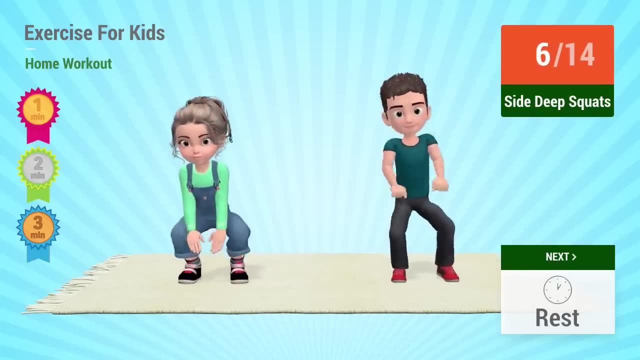 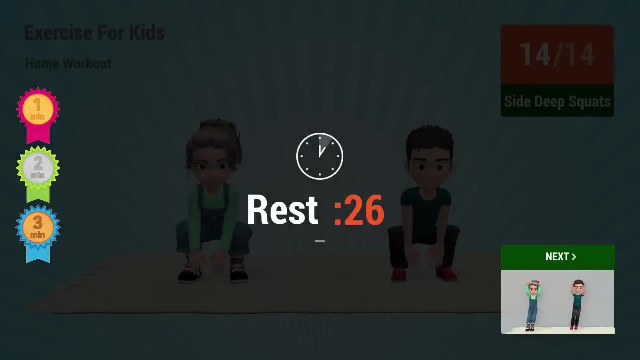 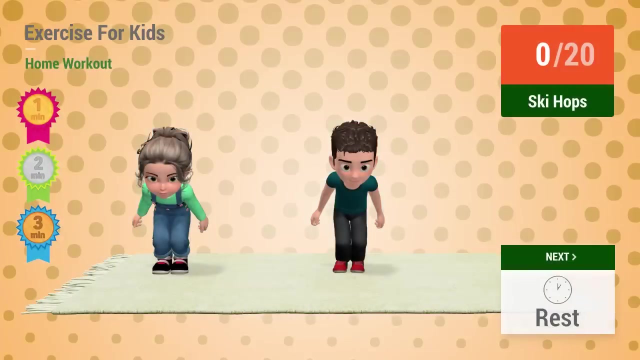 two, three, two, one go one two side deep squats in five, four, three, two, one go one, two, three, four, five, six, seven, eight, nine, ten, eleven, twelve, thirteen, fourteen. Rest time Up next. Ski Hops. in five, four, three, two, one go one. two, three, four, five, six, seven. 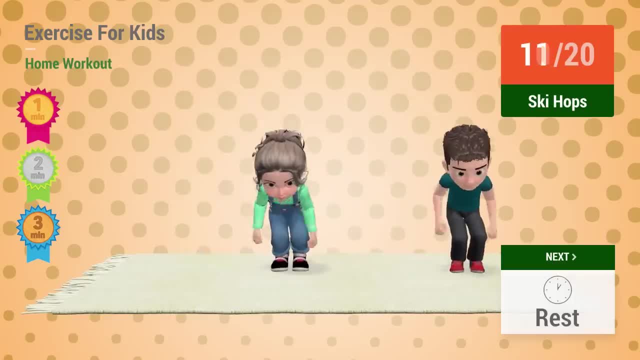 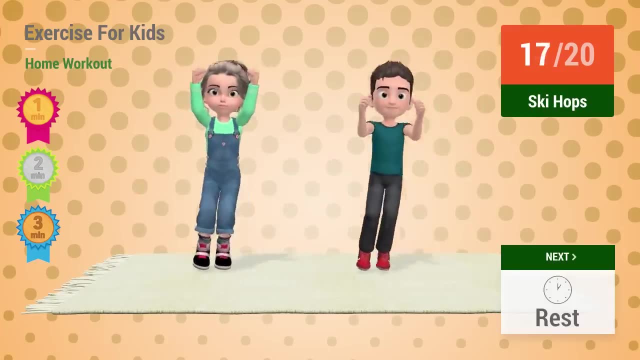 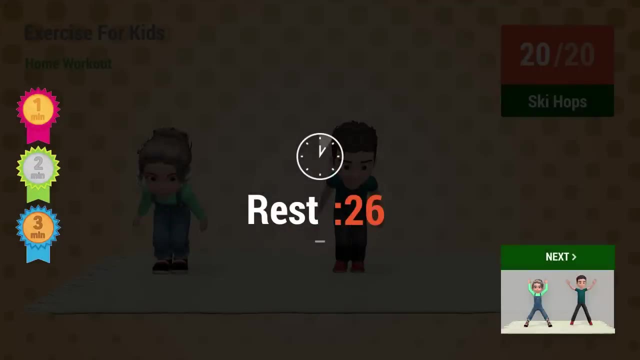 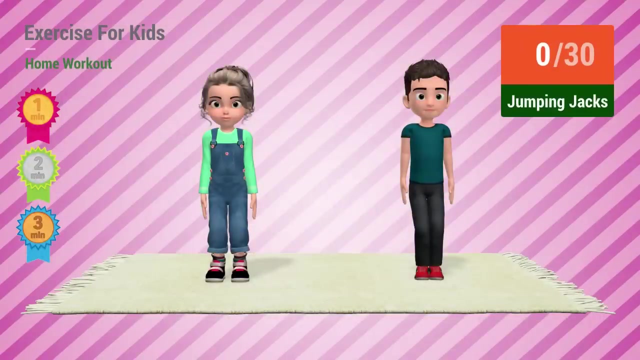 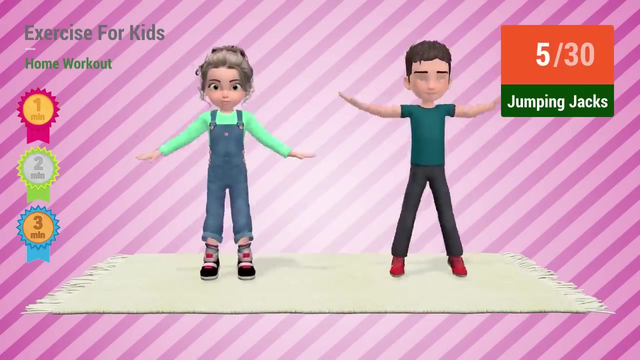 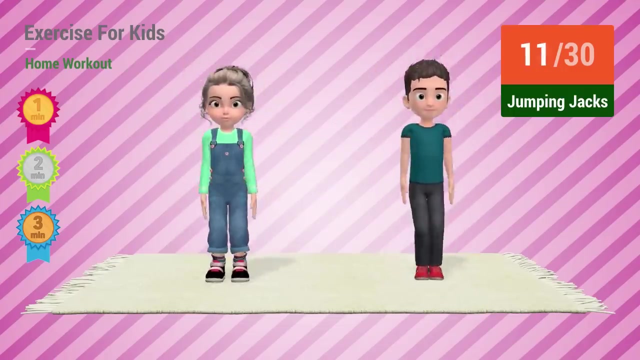 eight, nine, ten, eleven, twelve, thirteen, fourteen, fifteen, sixteen, seventeen, eighteen, fifteen, nineteen, twenty Rest time Up next Jumping Jacks in five, four, three, two, one go. one, two, three, four, five, six, seven, eight, nine, ten, eleven, twelve, thirteen, fourteen, fifteen, sixteen, seventeen, eighteen, nineteen. 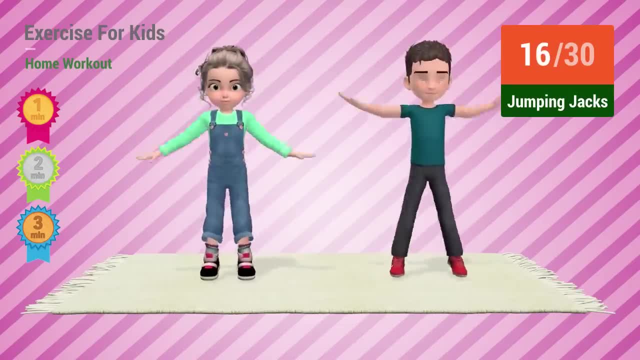 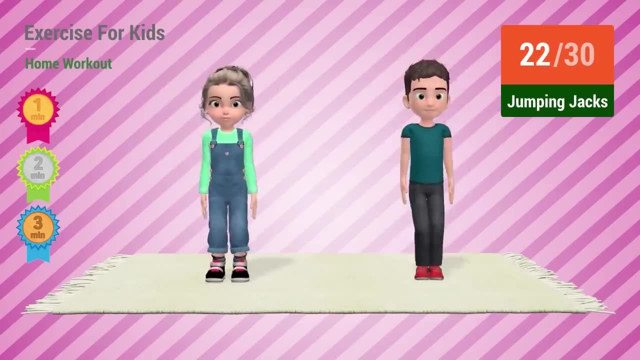 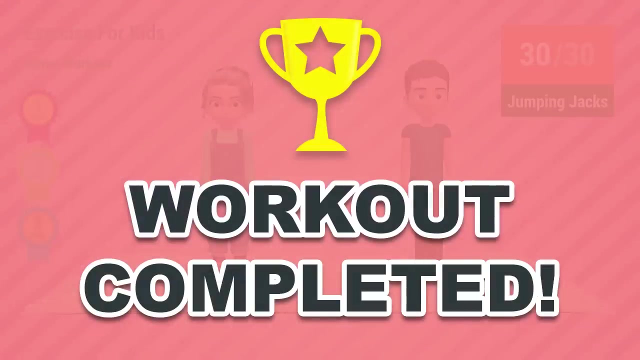 twenty Rest time. Up next Squat Triceps in five: four, three, two, one. go one, two, three, two, one, go one, two, three, two, one, two, one jump Rest time". Congratulations, You've successfully completed this workout. Please subscribe to the channel.